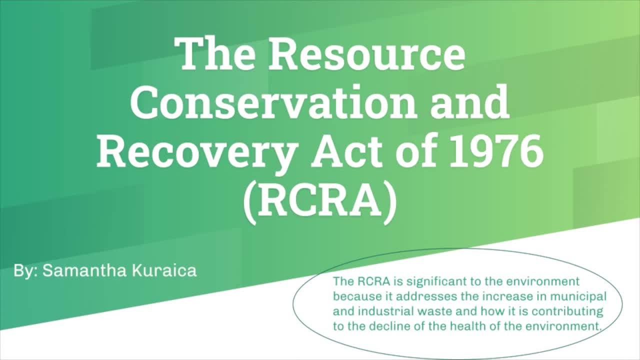 Hello, my name is Samantha Karayka and I'm going to be talking about the Resource Conservation and Recovery Act of 1976, also known as the RCRA. I chose this legislation because it's significant to the environment. It addresses the increase in all the industrial waste all across the nation and how it's contributing to the decline of the health of the people and the environment. 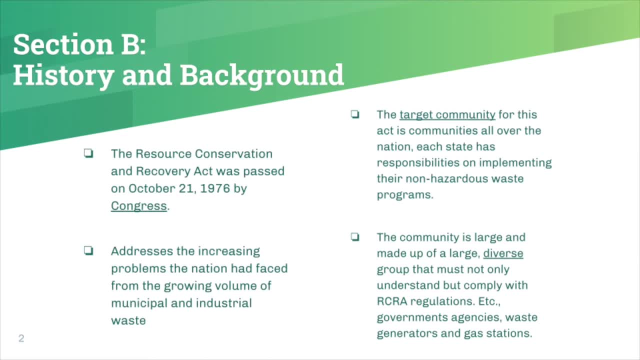 And some history and background on this legislation. The Resource Conservation and Recovery Act was passed on October 21st of 1976 by Congress And again it addresses the increasing problems the nation has faced from the growing volume of all the municipal and industrial waste. 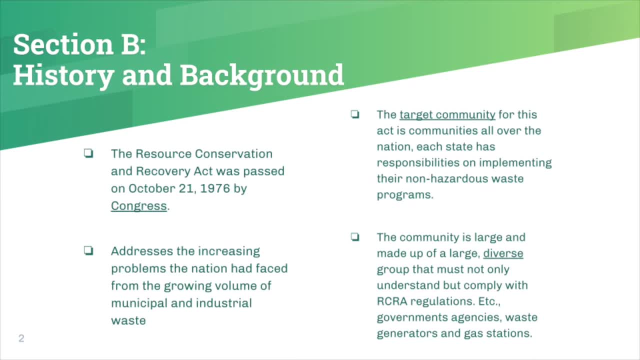 The target community for this act is really all the communities all over the nation, as each state has contributed a lot to all the hazardous waste. Each state has its own responsibilities on implementing their non-hazardous waste programs, And the way that this influences cultural implications is: the community is large and made up of diverse groups that must not only understand but also have to comply with RCRA regulations. 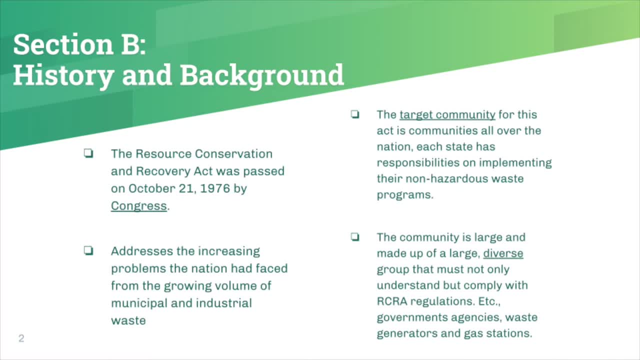 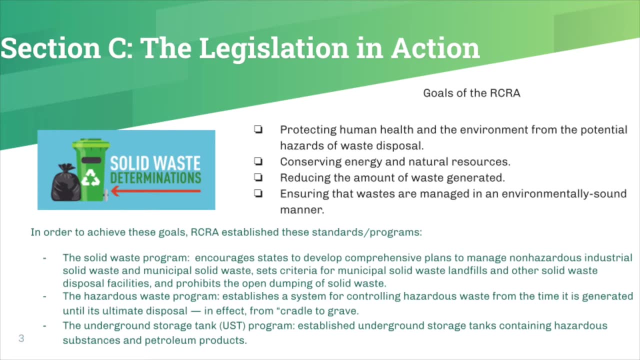 These include government agencies, waste generators and gas stations. Alright, so now we'll talk about the legislation in action. Some of the goals of the RCRA- These are coming from directly their website- are to protect human health and the environment from potential hazards of waste disposal, conserving energy and natural resources, reducing the amount of waste generated and ensuring that wastes are managed in an environmentally sound manner. 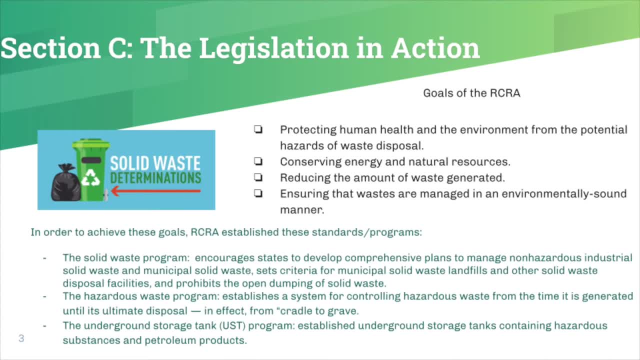 So, in order to achieve these goals, the RCRA also established some standards and programs, some of which include the Solid Waste Program. So what this does is it encourages states to develop their own plans to manage their non-hazardous industrial solid waste, and they set criteria for those wastes- things like landfills and disposal facilities- and it prohibits the open dumping of solid waste. 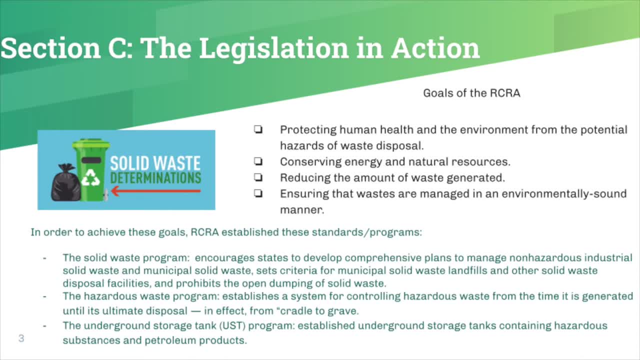 Another program is the Hazard Waste Program, and this establishes a system for controlling hazardous waste from the time it is generated until the time of its disposal. So basically, what they call it is cradle to grave from start to finish. And the last one is the Underground Storage Tank. 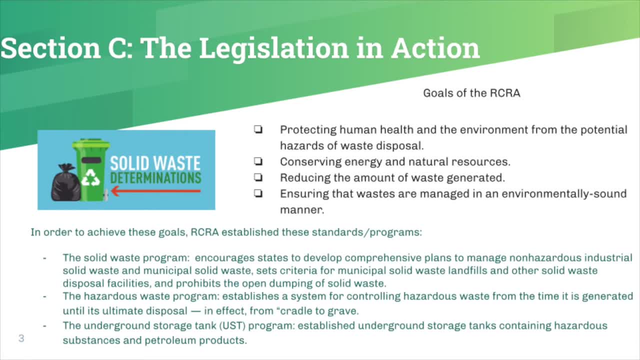 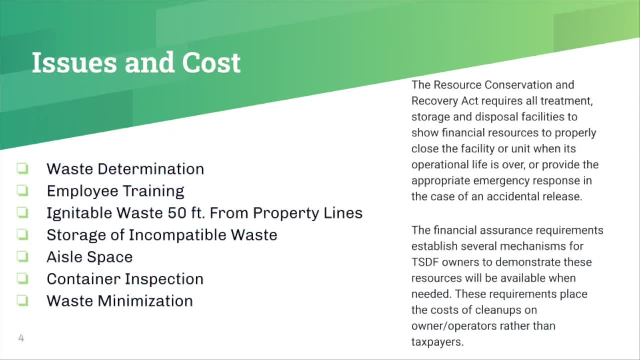 UST program, and this establishes underground storage tanks containing hazardous substances and petroleum products. So now discussing issues and costs. There are some issues that come with the RCRA, some of them being waste determination, employee training and with waste determination, These are things like determining if the waste is even hazardous, So the process of providing safety data. 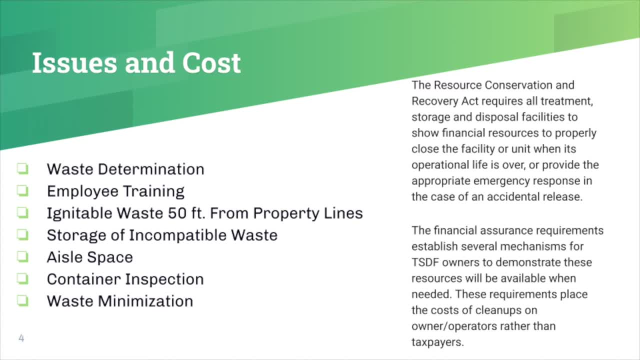 And above the data sheets. And then employee training would be making sure that all the employees who are responsible for disposing of hazardous waste are properly trained on how to. And then some other issues are storage of incompatible waste, aisle space, container inspection and waste to minimization. 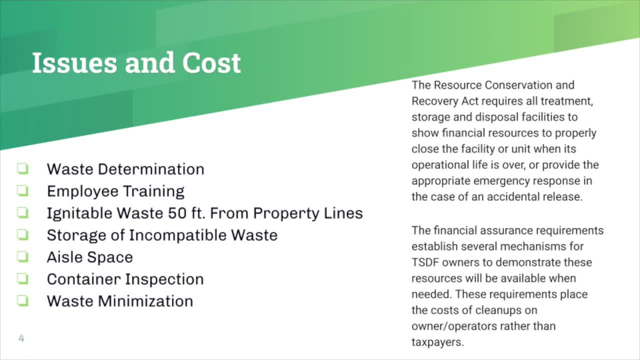 So for the cost. the Resource Conservation and Recovery Act requires all treatments, storage and always Kolleg equipment to meet the Utility, talkin' hourues and disposal facilities to show financial resources to properly close the facility or unit when its operational life is over or they want to be able to provide the appropriate emergency. 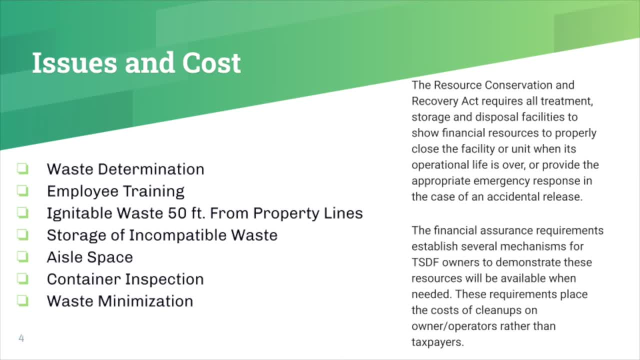 response in the case of an accidental release, and then when it comes to financial assurances, they require several mechanisms for all of the owners to demonstrate that these resources will be available when needed, and ultimately, this puts the costs of cleanups on owners and operators rather than taxpayers of the community. now moving on to regulations and 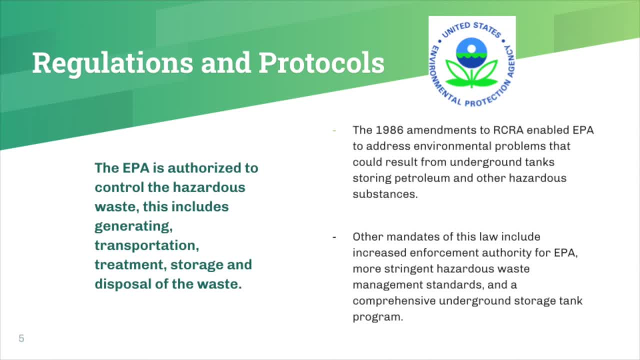 protocols. so the rcra is under complete control of the epa or the environmental protection agency. the epa is authorized to control the hazardous waste, again, from crate to grave meaning, from generating transportation, treatment, storage and disposal of the waste. and in 1986 the amendments: 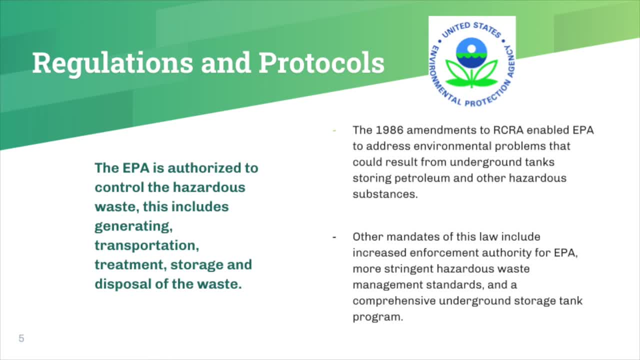 of the to the rcp or a enabled epa to address environmental problems that could result from the underground take storing petroleum and other hazardous substances. and some other mandates of this law include increased enforcement authority for the epa, more stringent hazardous waste management standards and a comprehensive underground storage tank program. 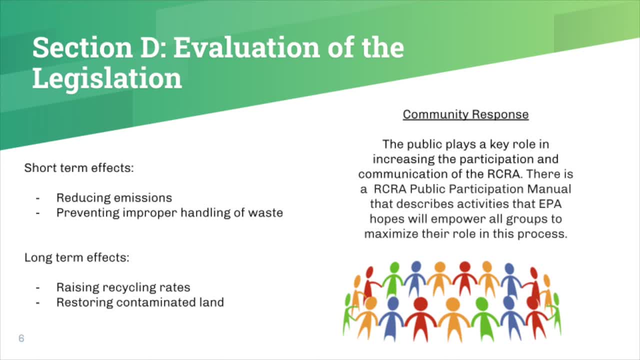 so now we are evaluating the legislation. some of the short-term effects of the rcra are that they have reduced emissions and they've prevented improper handling of waste, and some of the long-term effects are they have been able to raise the recycling rates all across the nation, and they've also been able to restore. 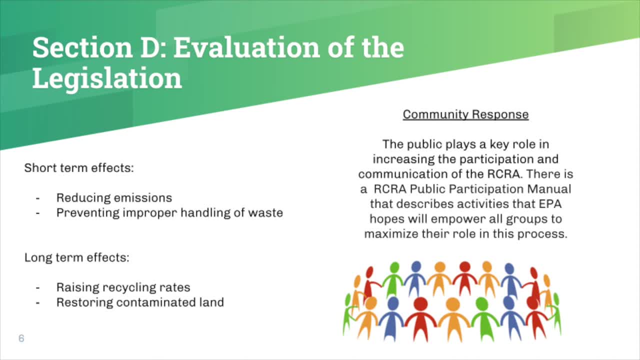 contaminated land as part of the community. some of the responses. so the public plays a key role in increasing the participation and communication of the rcra. the community has been shown to increase its activities in the rcra and then the rcra created a public participation manual that 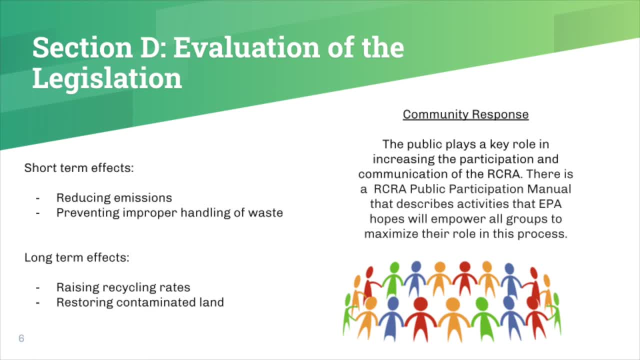 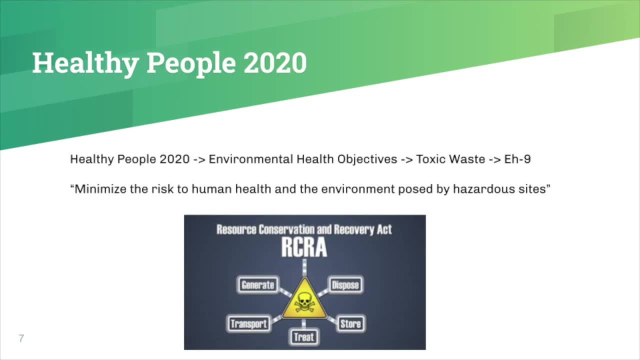 describes all of these activities that the epa hopes will empower all groups to maximize their role in this process as part of the healthy people 2020 agenda. under environmental health objectives and toxic waste: eh-9 quotes: minimize the risk to human health and the environment. posted by. 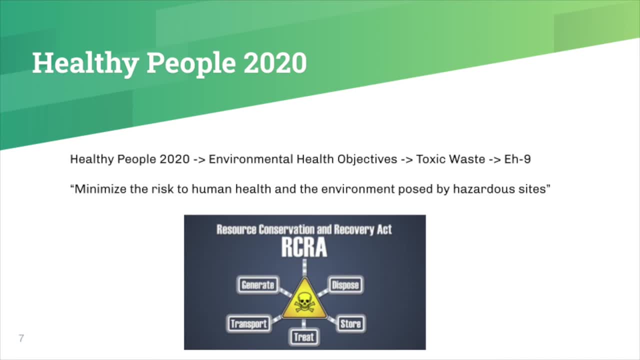 hazardous sites topic directly correlates to the RCRA, because the RCRA strives to minimize the waste and, in collaboration with Healthy People 2020, are trying to reduce toxic agents from the environment and, in return, create a healthier environment for the community and the people. So now, in conclusion, I 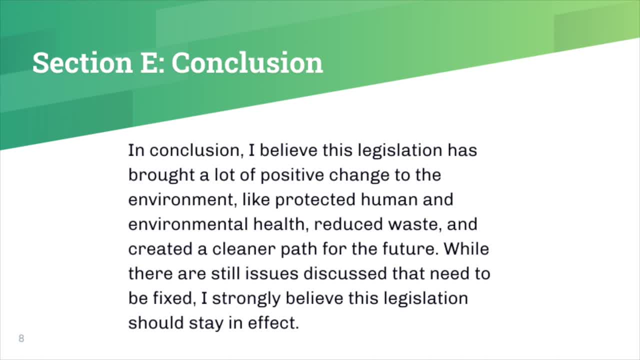 believe this legislation has brought a lot of positive change to the environment. It's protected human and environmental health. it's reduced waste and created a cleaner path for the future. while there's still a lot of issues, like we discussed earlier, that need to be fixed, I 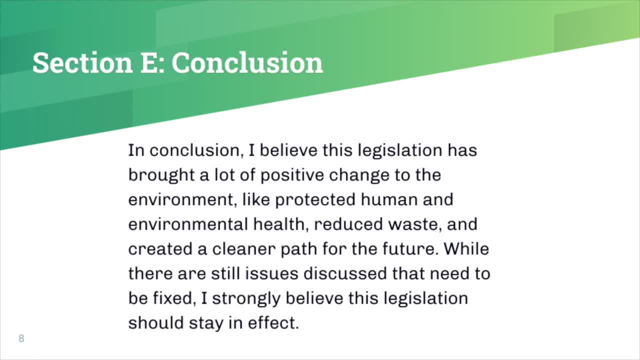 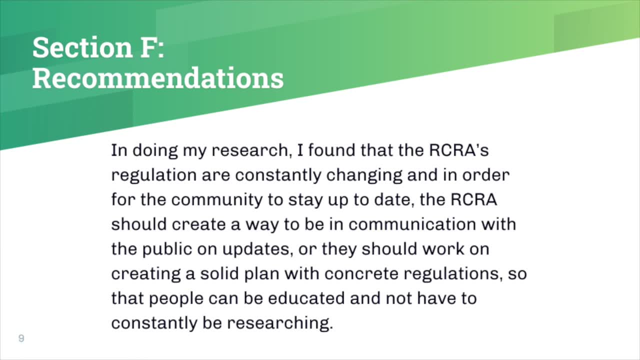 strongly believe that this legislation should stay in effect. Some recommendations I would give. while I was doing my research, I found that the RCRA regulations are constantly changing and updating and in order for the community to stay up to date, the RCRA should create sort of like a way to be in. 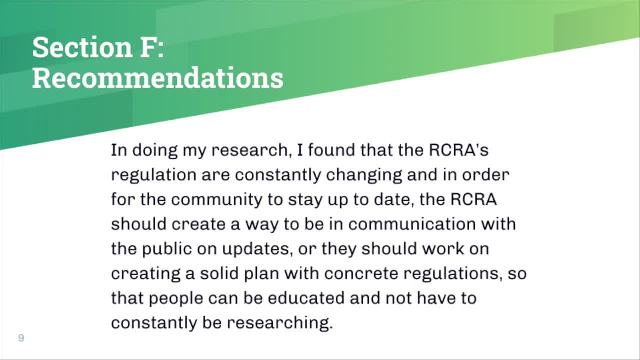 communication with the public on any updates. or, if they aren't able to do that, they should work on creating a better environment for the community, creating a more solid plan, one that's a little more concrete with its regulations, so that the people can be thoroughly educated and they wouldn't have to be constantly checking. 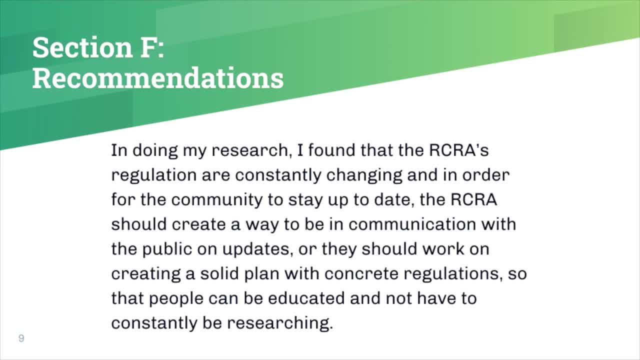 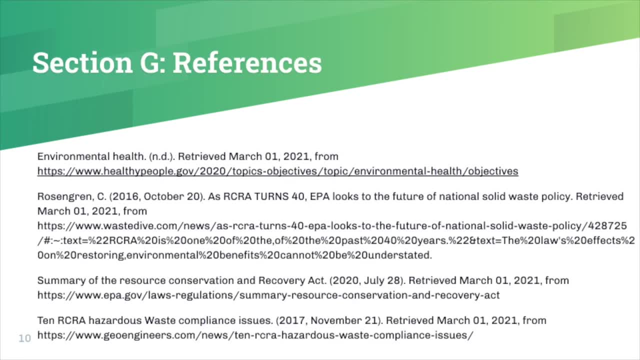 websites or posts about updates, and they can just continue to follow one set of regulations. And that is it for my RCRA presentation. These are my references and thank you very much.